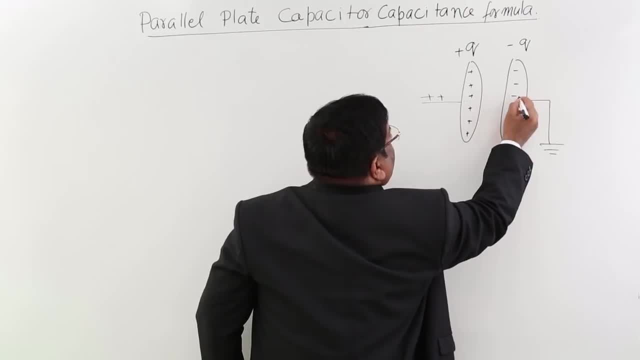 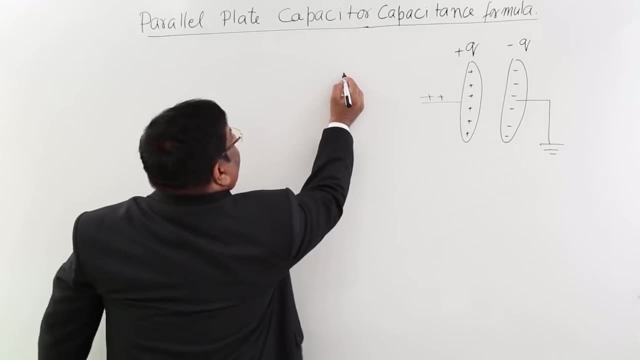 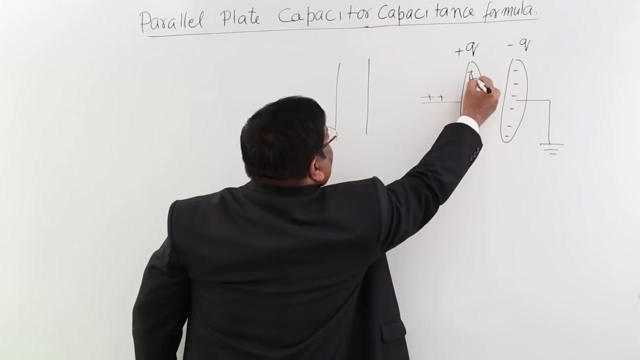 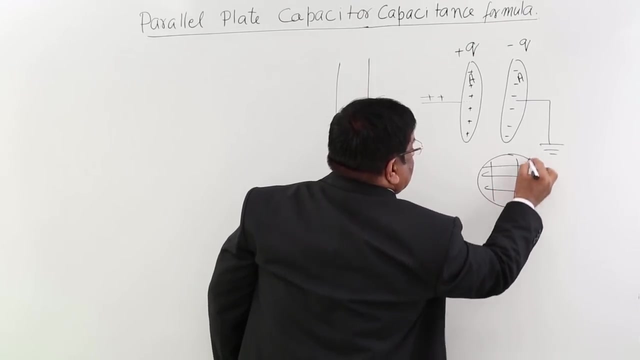 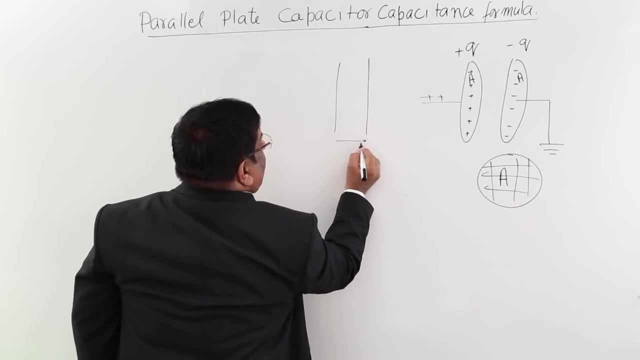 this carries minus q charge. Remember, charges are always equal. If this I make it this way simple, then these two have got area A, that is, this area. this total area is A. Now I see it in this way, the distance between the two plates is d. 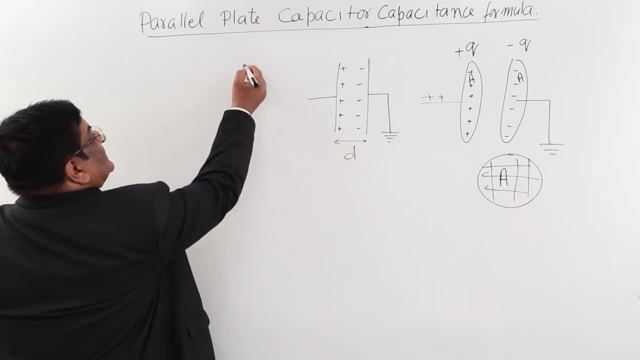 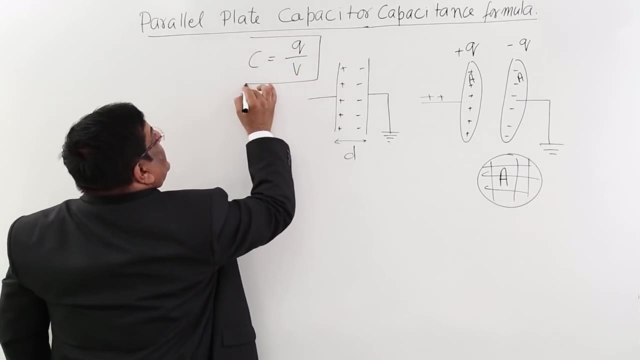 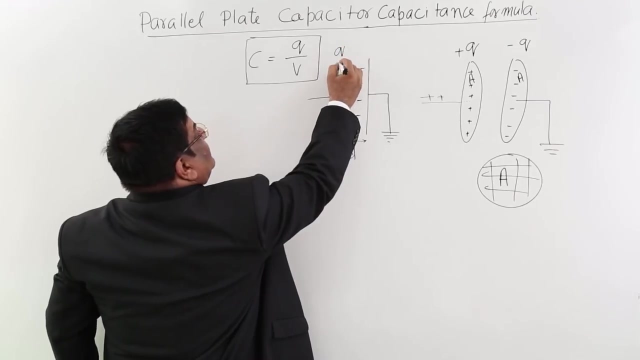 Now I want to calculate capacitance or for capacitance. I have only one formula: that C is equal to q upon V. I want to calculate both the things and I have given it charge q. If I give it charge q, then I want to calculate what is. 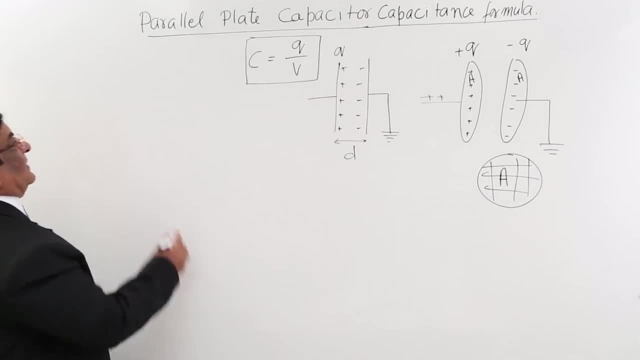 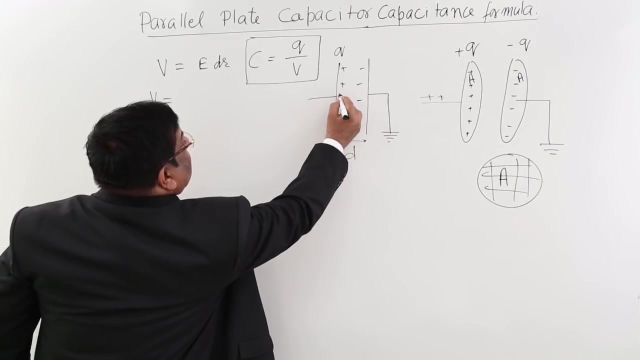 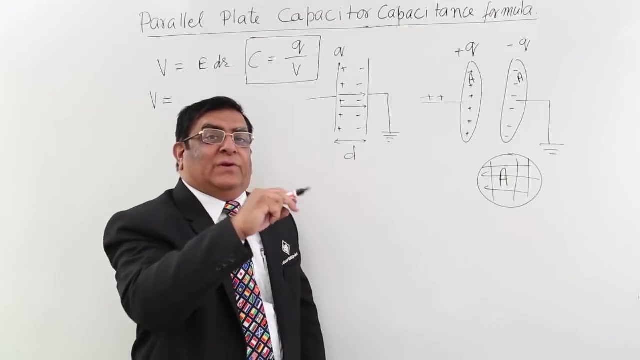 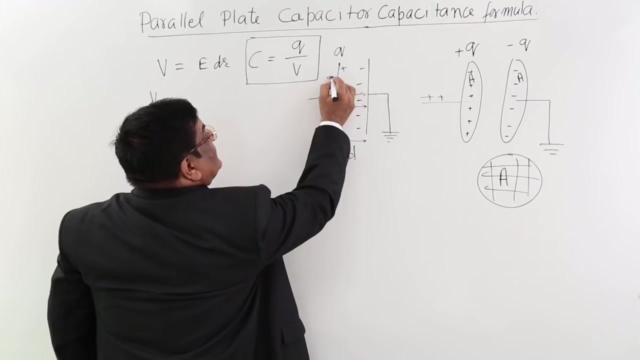 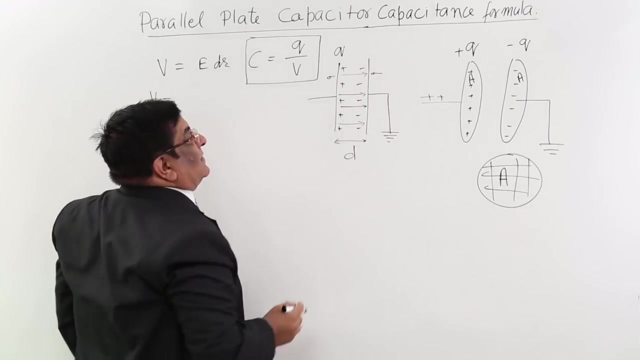 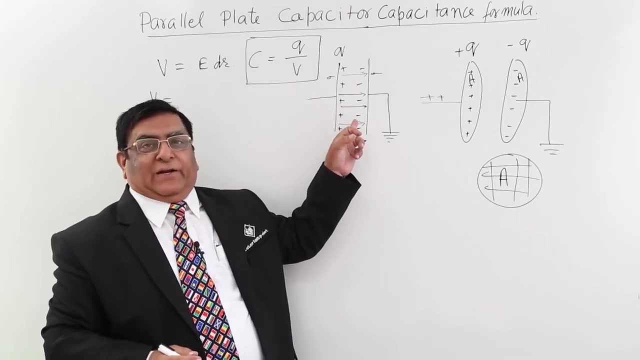 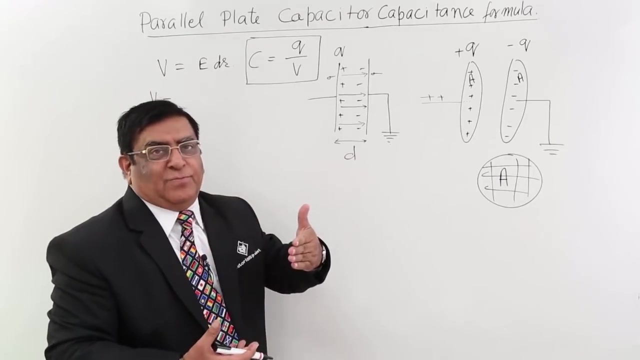 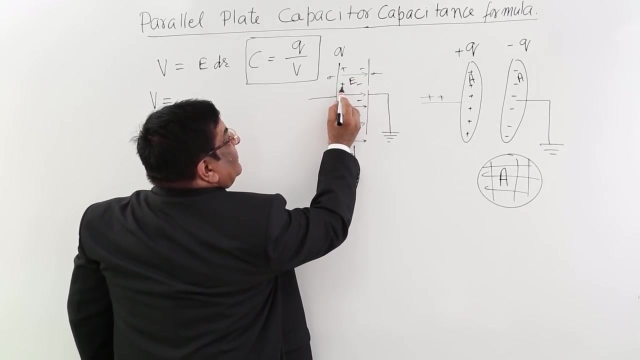 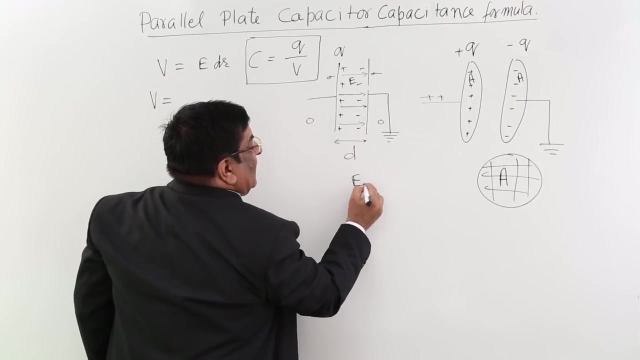 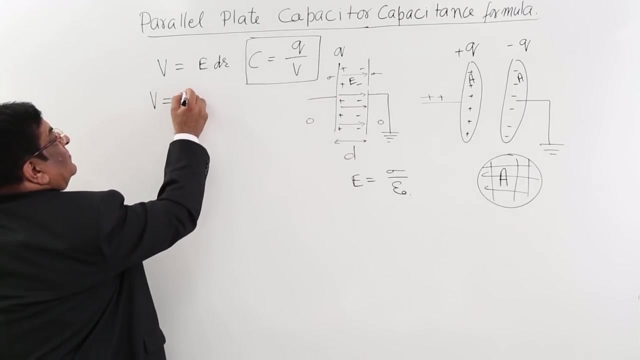 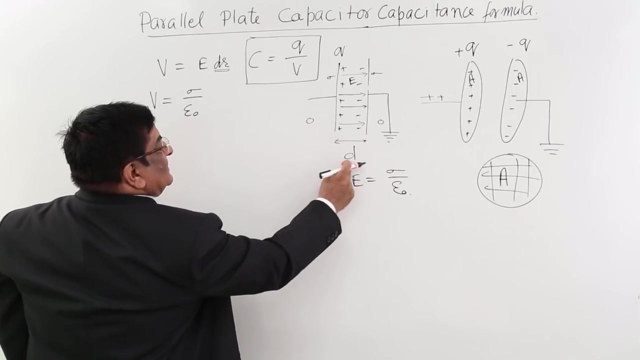 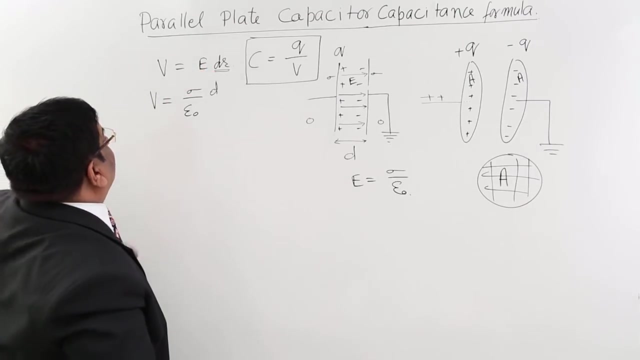 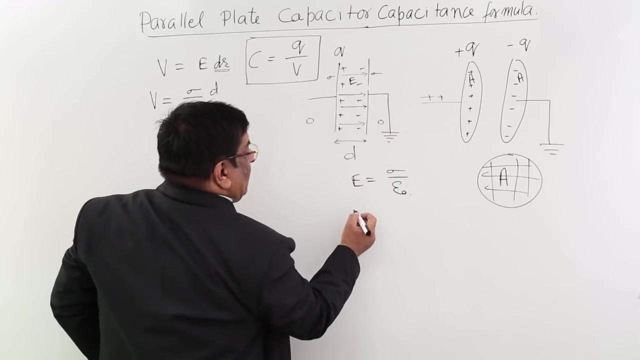 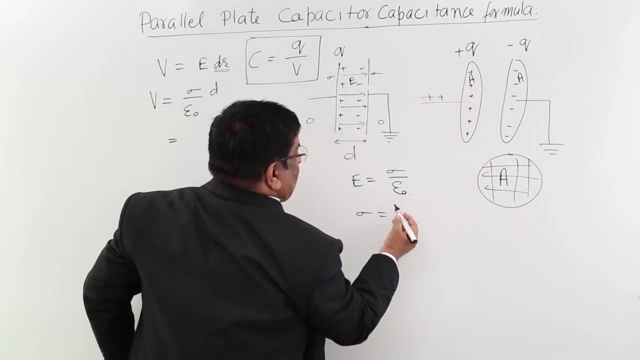 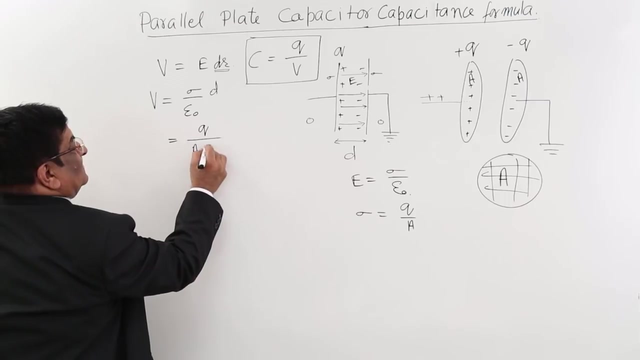 the potential difference here. For potential difference calculating we have a formula: V is equal to E into dr. This, you remember, I have calculated by total charge on this plate, that is q and divided by area, q upon area. So now I can write it: q upon area multiplied by d. This is value of potential. If this 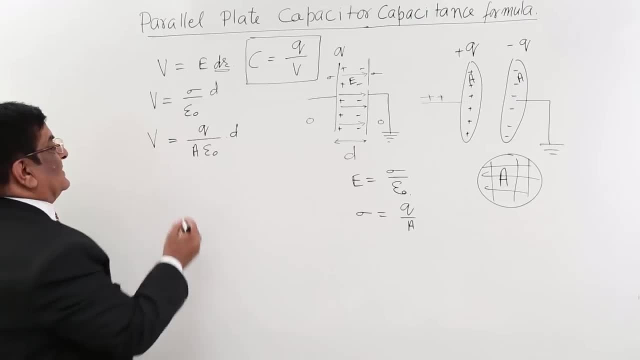 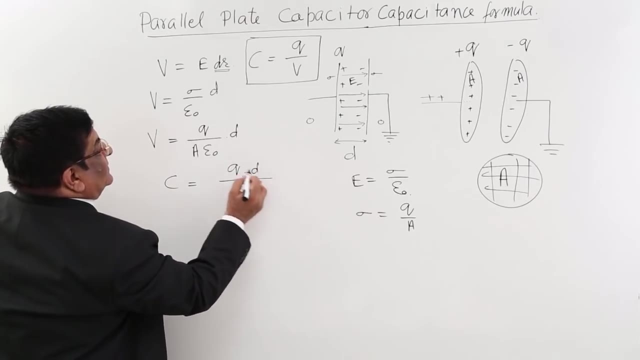 is value of potential difference between the two plates, then this capacitance. capacitance is equal to q into d upon area. The left side looksрg çf선 is equal to принцип Pastor addingg Sorry, from top or bottom. 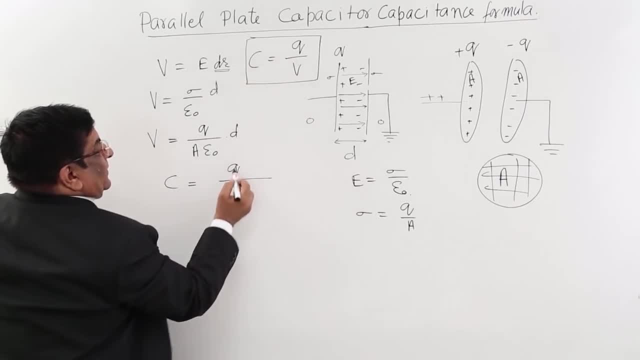 That is sorryprocess, something untruth, And this is part of that. So let us put some r and let us put some the energíae Right, this is a condenser, So I have selected these two accidents and I have already calculated r. 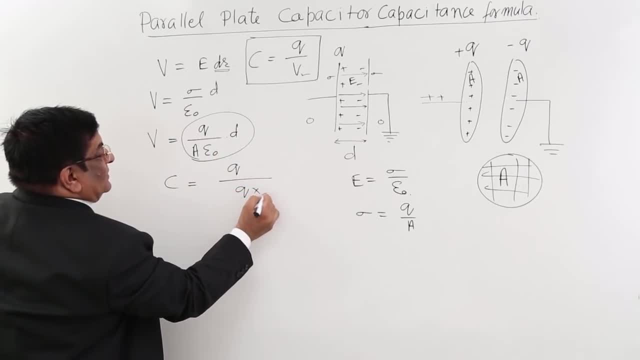 So I will write such these two problems, A and d. That is sorry. potential is equal to q upon q upon V. This V I place from here, And this is q into d, upon A epsilon naught. So this qq is cancDAble plus 1.. 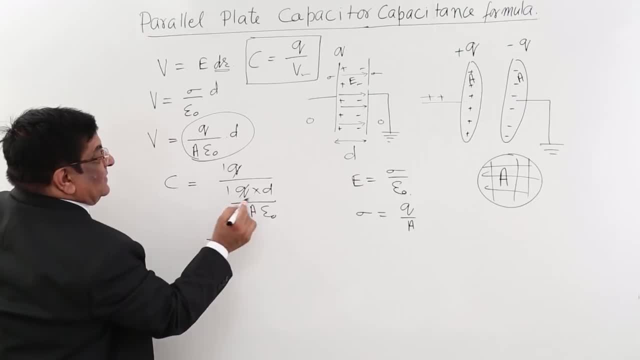 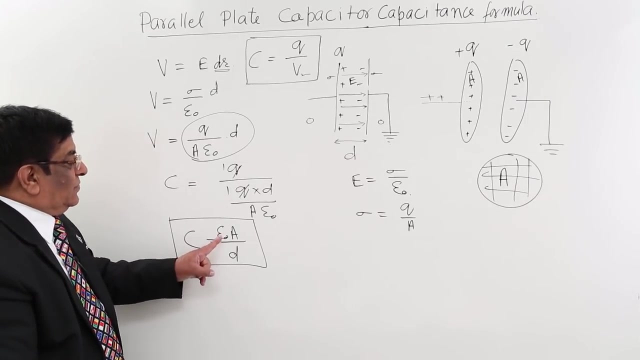 A epsilon naught. So this q is cancelled and what we get? it? epsilon naught A upon D And if I put peaceful bliss equation, He cannot get things. Sure, He cannot get them d. this is capacitance, very simple relation capacitance is equal to. this is medium, whatever. 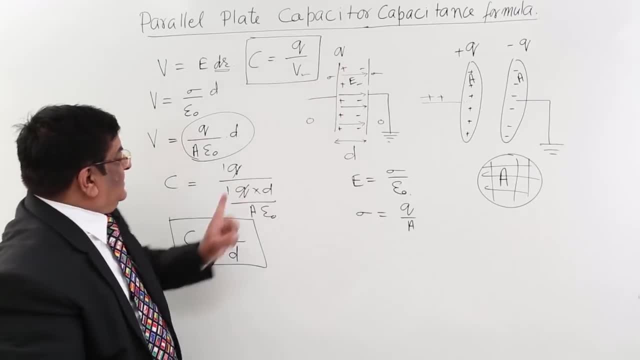 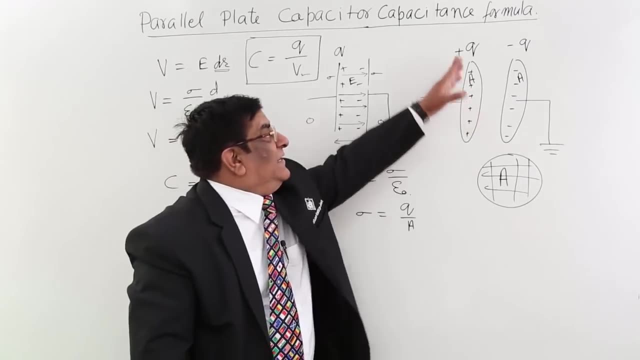 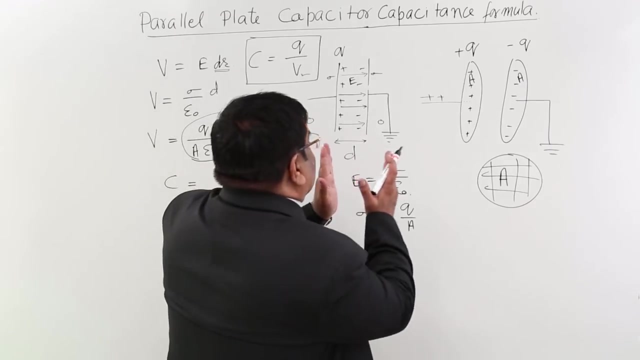 is the medium between the two. if it is free space, this is epsilon, not area of the plate and distance of the plate. larger is the area, larger is the area, larger is capacity, but nearer is the distance. if this distance decrease, the capacitance increase. why it happens. if 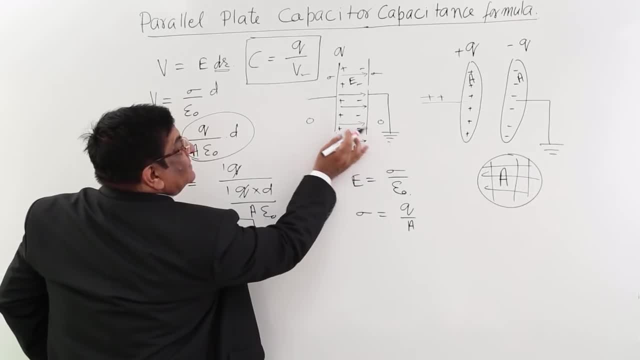 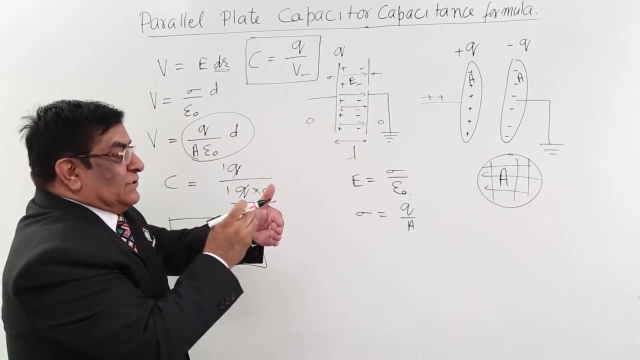 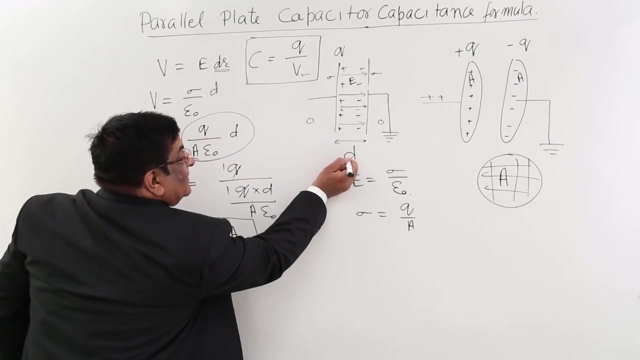 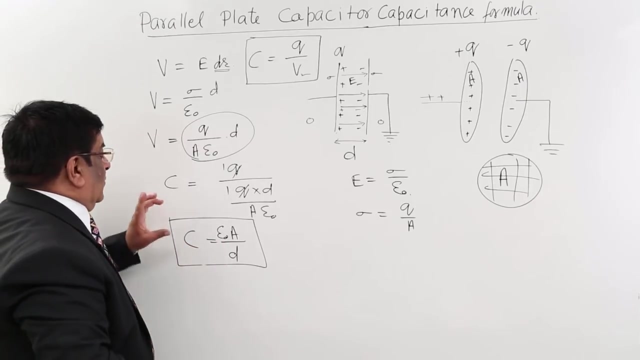 distance is small, then the charge attraction will be more. induction will be more. if this distance is small, the force is more. induction is more, more charges will come and the binding force will be more. therefore, if d decrease, the capacitance or the charges will increase. so this is our fundamental formula for capacitance of a parallel plate capacitor. 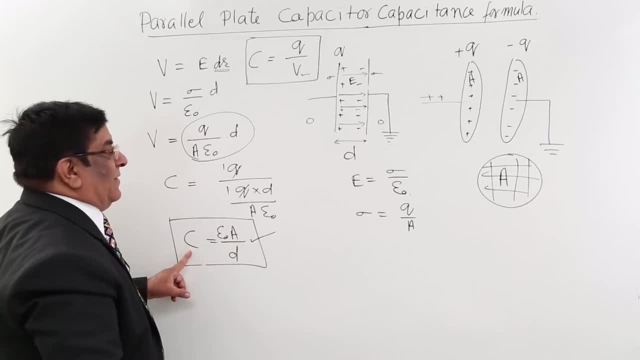 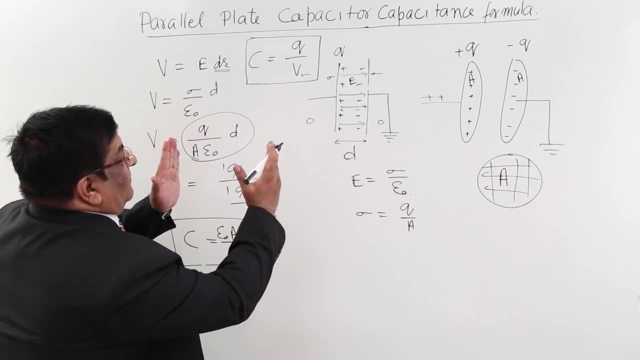 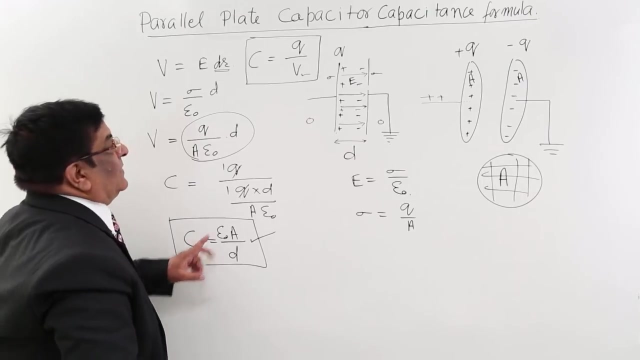 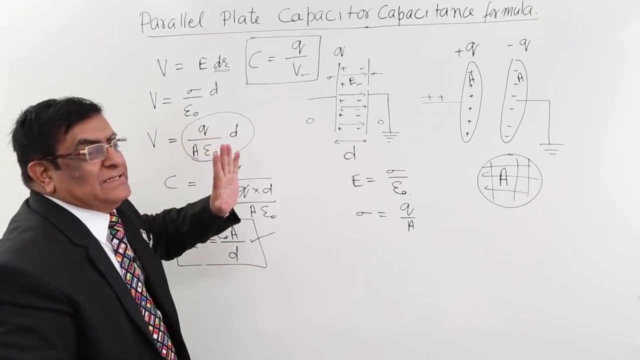 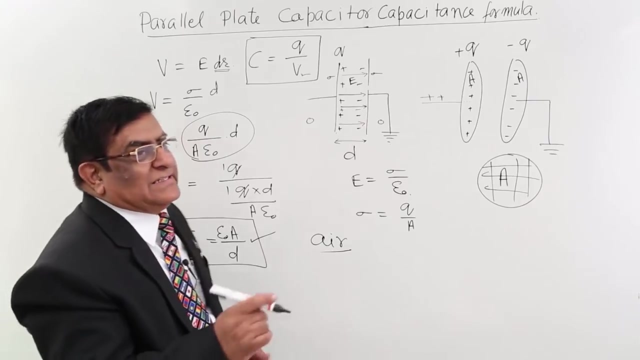 remember it: larger area, larger capacitance. the closer it is, then capacitance will be large. and if you make them away, away, away, the capacitance will go on decreasing. so this is fundamental formula of capacitance and between the two plates at present there is there is a free space or there is air. ok, so now in the next lecture we will see if we